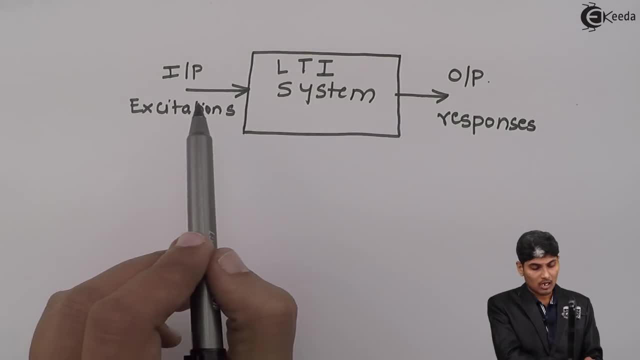 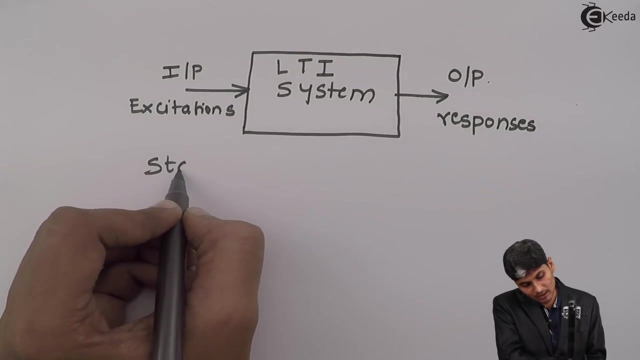 my output cannot be determined. So I will give a known input and based on this known input I will characterize what type of system is this? So, to characterize a system, I will have set of inputs and set of outputs. So the known or the standard inputs that I will be applying is standard inputs that will be applied. 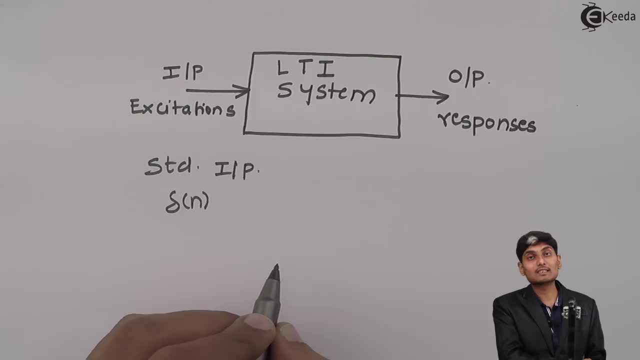 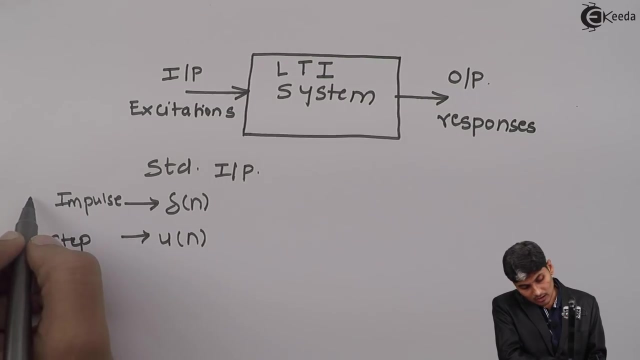 will be delta of n, which is impulse, And u of n, which is step. So I have a signal called impulse and I have a signal called step. Specifically, they are unit impulse and unit step. So the height is one. So I have a unit impulse. 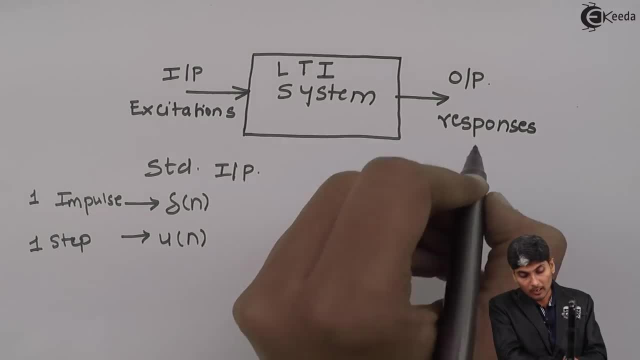 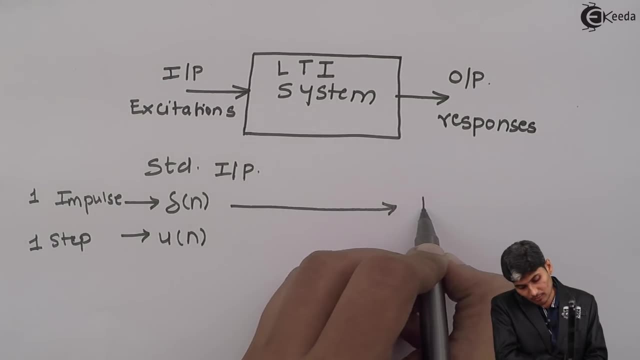 or I can apply as unit step, And the response that I get based on this is called as impulse response, which is denoted as h of n. We have seen this term, h of n, previously. I called this as a signal before, But this is actually a response, And which type of response is this? This is called. 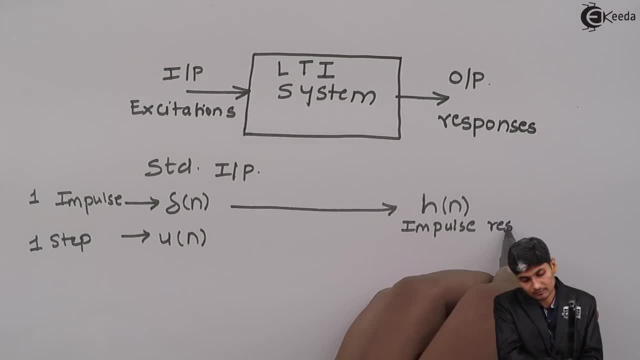 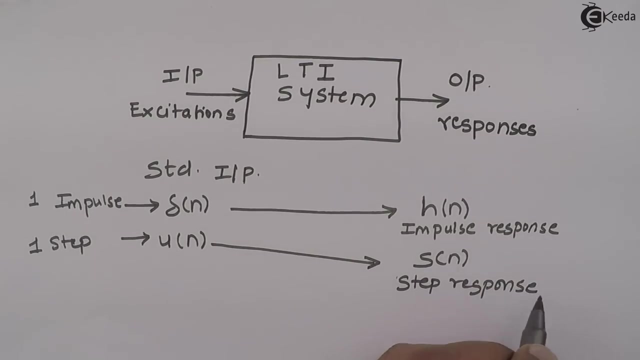 as impulse response. And when I give an input as u of n, then the response that I get is called as s of n, which is called as step response. So when I give input as delta n, that is impulse, the output which I get is called as a impulse. 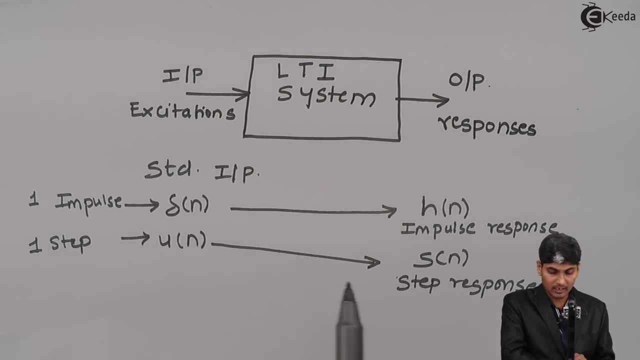 response, The input. if I give u of n, then output is s of n or step response. So my output over here. normally we denote using y of n. So now my y of n is equal to h of n and here y of n is equal. 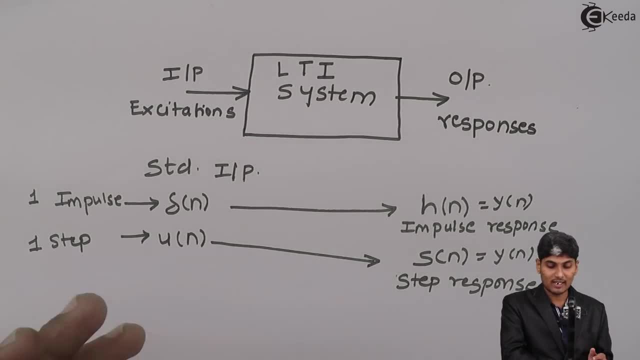 to s of n. So I will have set of inputs, That is, x of n, and set of outputs, which is y of n, which will characterize the system. So whenever I represent a system, I will take set of inputs and I will give set of outputs. 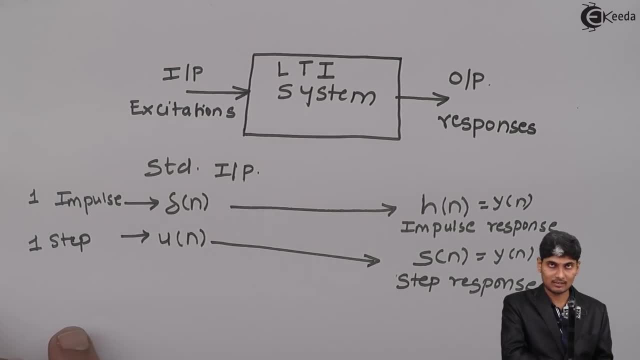 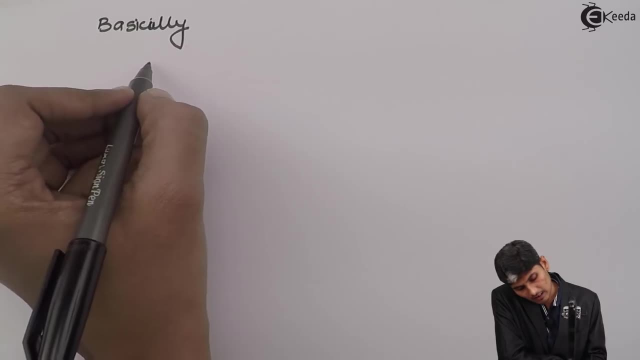 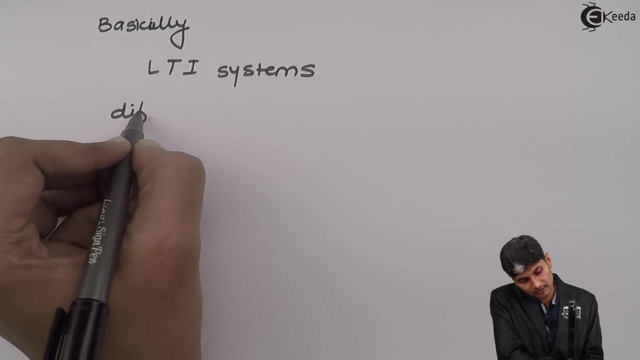 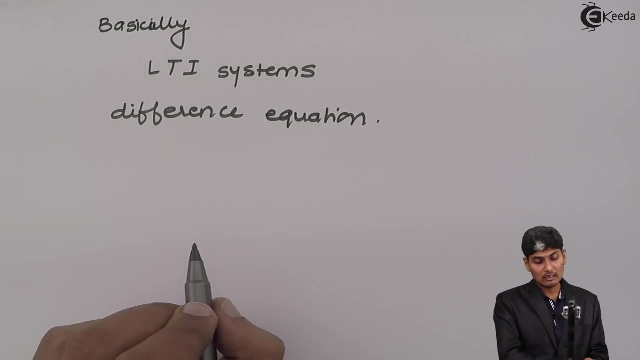 And that can be helped as getting a characterization of a system or representation of a system. Basically, LTI systems are represented using difference equation. What do you mean by difference equation? A difference equation is similar to that of differential equation, But differential equation is used for representing a continuous time signal, whereas difference equation is used to represent a discrete time system. 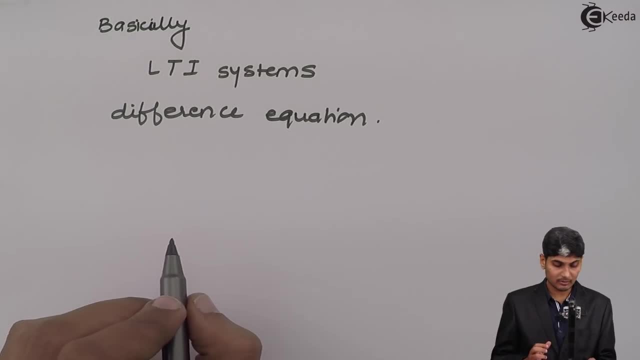 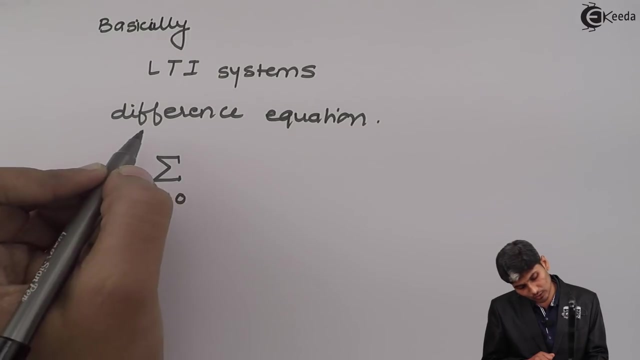 As we have seen that the characteristics of a system is given by set of outputs and set of inputs, So difference equation will have a set of outputs and set of inputs and relation. So the difference equation in general is given. as summation, k is equal to 0. to let us 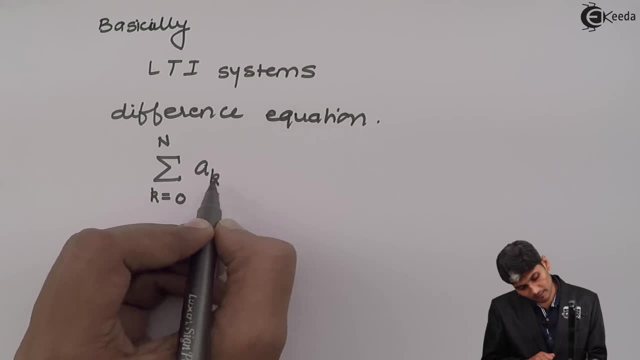 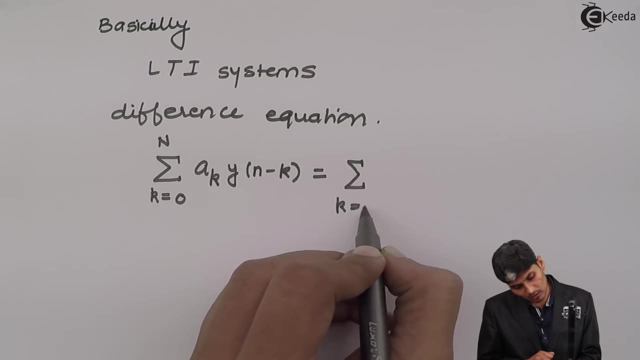 say n: okay, financiate k. x of n minus k equals to summation k k going from 0 to m. this is your comma: bk x of n, MICHAEL, SHORT Of x minus 1. k. so now we have a set of, or a relation between the set of outputs and set of inputs. now why i'm 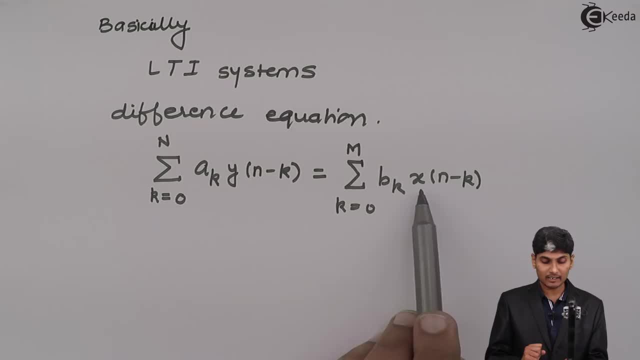 saying set of outputs and set of input is because i'm writing here x of n minus k and here also y of n minus k. what does it represent? is, if i put k is equal to 0, then i'll get y of n and x of n. 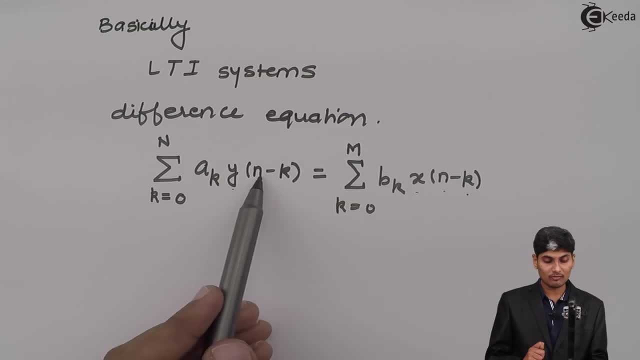 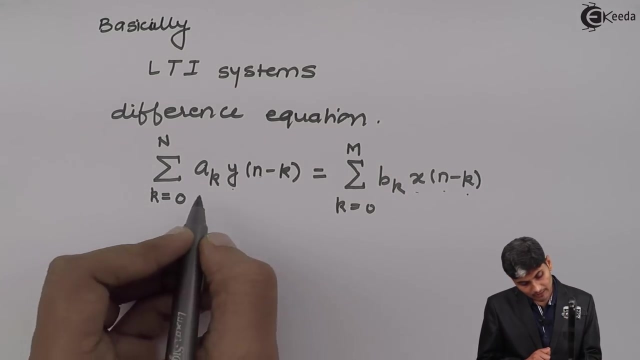 then i put: k is equal to 1, i'll get y of n minus 1, x of n minus 1, and so on. so i have all delayed version of y's, that is, outputs and delayed version of inputs. so we have, if i expand this equation, 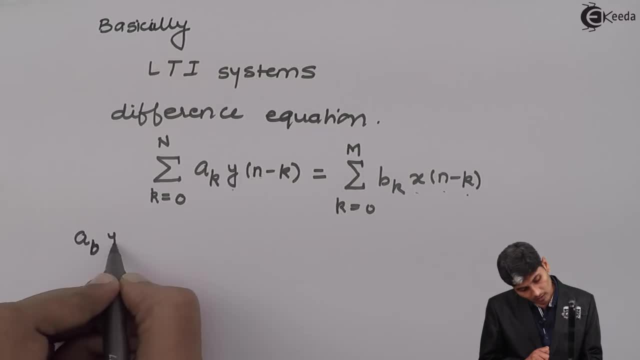 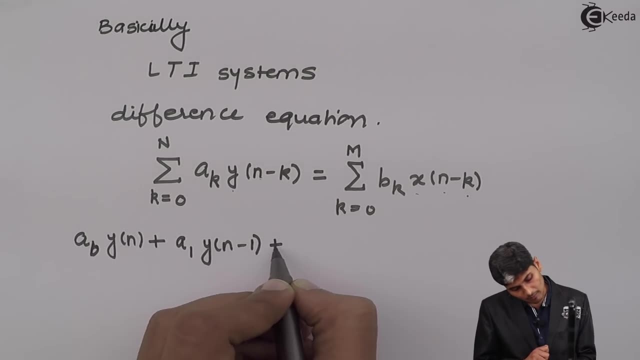 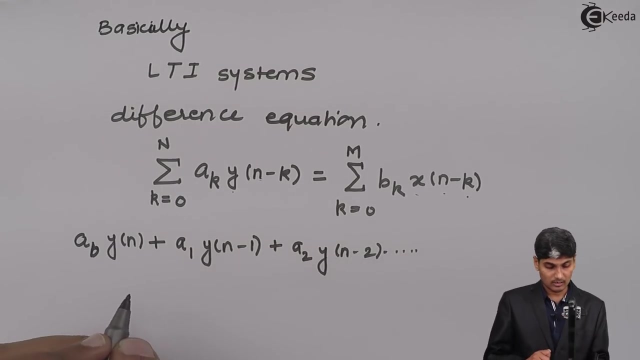 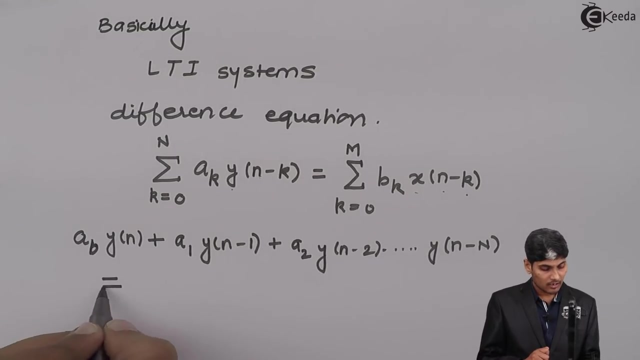 i'll get a, let us say 0 y of n plus a1, y of n minus 1 plus a, 2 y of n minus 2, and so on and so forth, till the last composite value comes as y of n minus capital. n equals to this. is this equal to sign? then i have b 0 x of n plus b 1 x of.